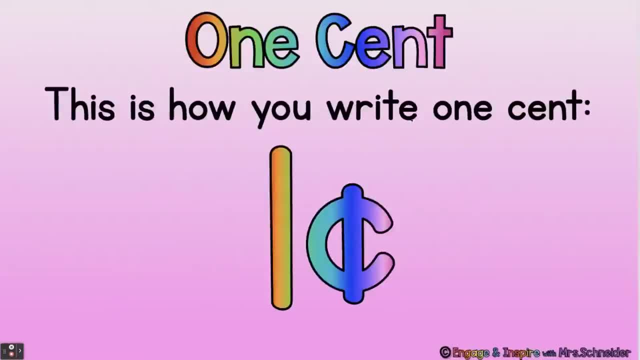 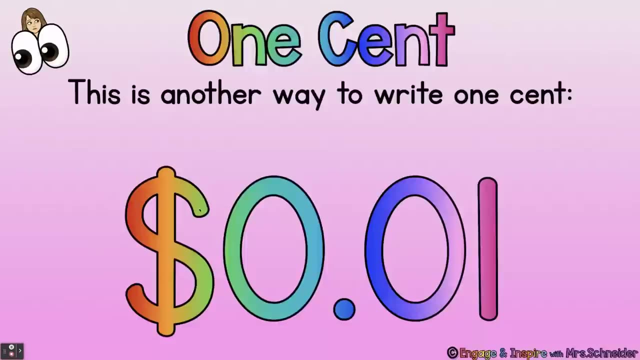 A penny is worth one cent. This is how you write one cent. This is a one And then a C with a line. This is another way to write one cent. This is a dollar sign, And you see dollar signs either with one line down the middle or sometimes two lines down the middle. 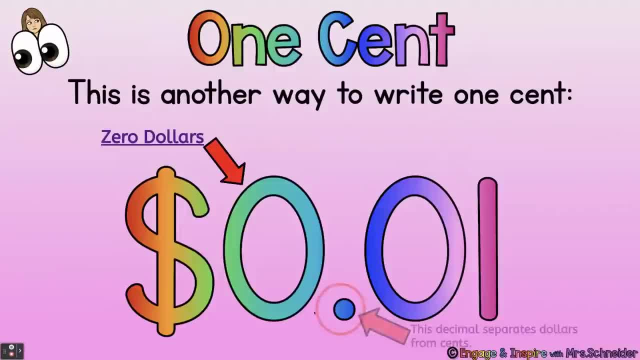 And the way that this is written. it means zero dollars, And then there's a decimal point right here which separates the dollars from the cents. And one cent. You know how we can write single digit numbers: zero one. Well, this is one cent. 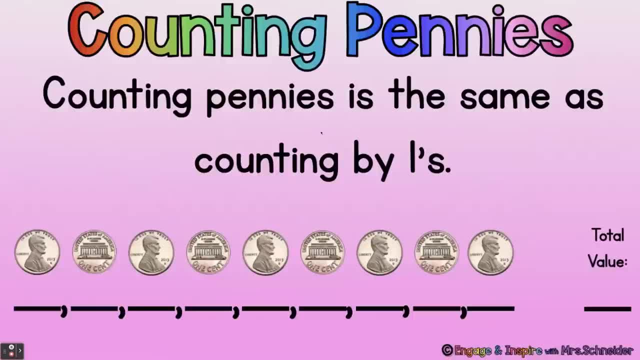 So zero dollars and one cent Counting pennies. Counting pennies is the same as counting by ones, So you go one and then you're adding one more. So one plus one is two, three, four, five, six. 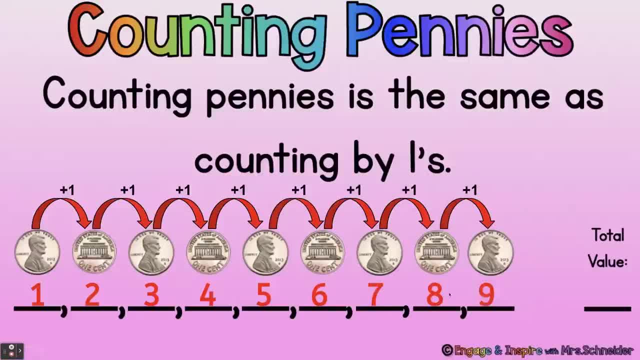 seven, eight, nine. So here we have nine pennies And they're worth one cent each. So we have nine cents. The total value of these pennies is nine cents. What do you think? Can you buy anything with nine cents? 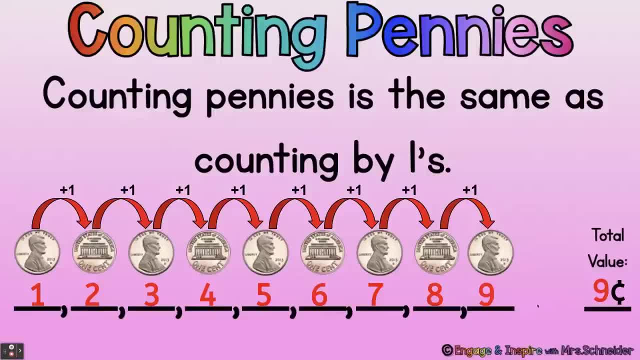 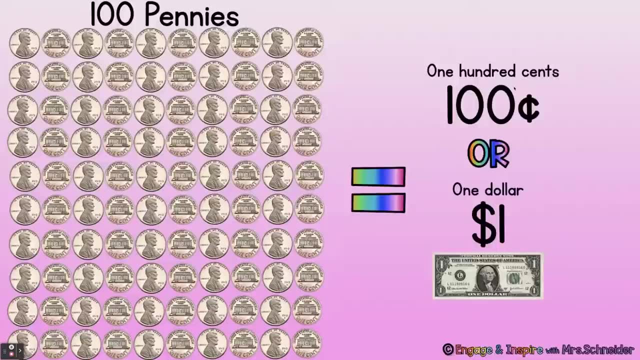 I haven't been able to. But my grandma said when she was little she got to go to the movies for only five cents. It only cost her five cents to get in the movies when she was little. One hundred pennies equals one hundred cents. 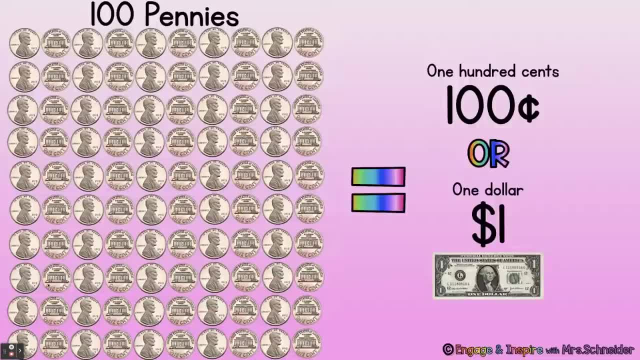 That's the same as one dollar, So you can trade a hundred pennies for a one dollar bill. That would definitely be a better choice for me, because I would probably lose all these pennies or they'd fall out of my pocket, And that would be a lot of counting. 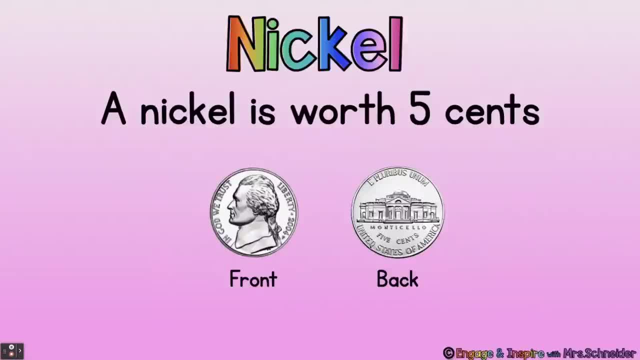 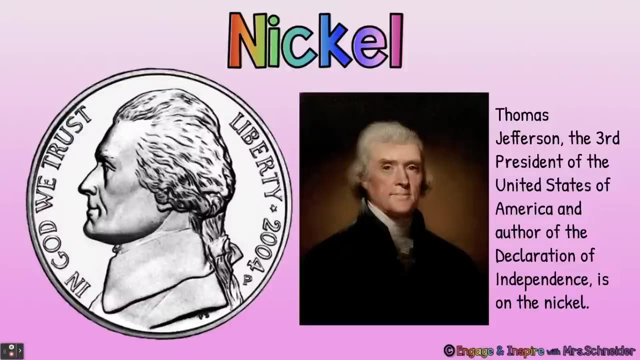 Sometimes it's just easier to have dollar bills- Nickel. A nickel is worth five cents. Here you see the front of the nickel And here you see the back of the nickel: Thomas Jefferson, the third president of the United States of America and author of the Declaration of Independence. 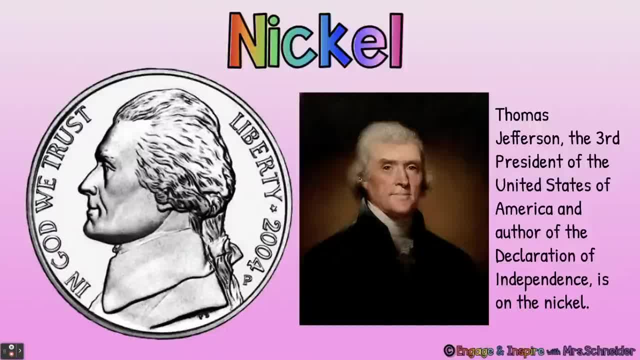 is on the nickel. What do you guys think? Does that look like him? I think it's pretty close And you know they all kind of had this long hair back then. On the back of the nickel is Monticello. 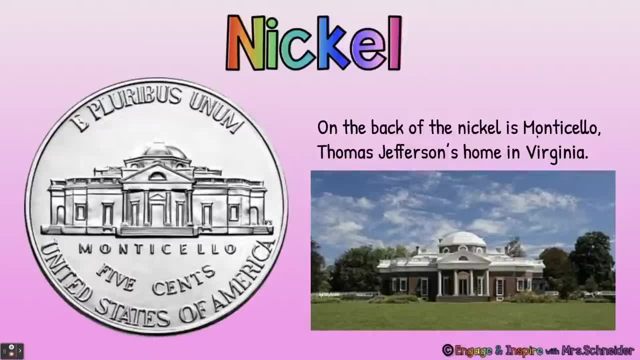 Or some people say Monticello, But it's an Italian word, So I'm going to say Monticello, Thomas Jefferson's home in Virginia, And actually you can take a tour of this home. If you went to Virginia, you can tour this home. 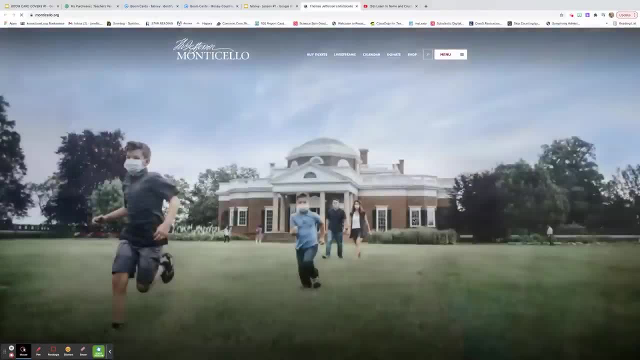 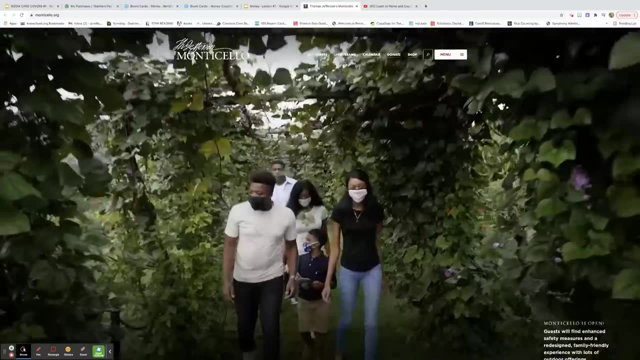 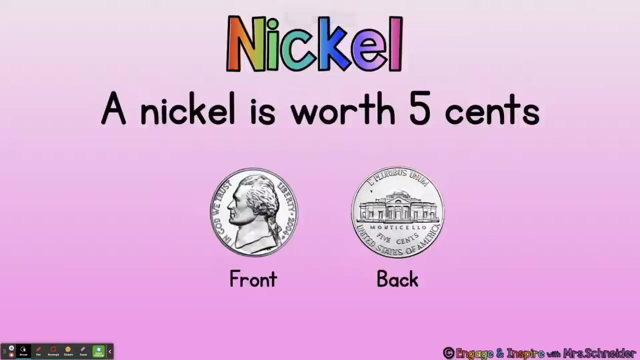 I'm going to click on it and show you. I included a link And here you see, this is Monticello And this is what is on the nickel. Isn't that fascinating. A nickel is worth five cents. Five cents. This is how you write five cents. 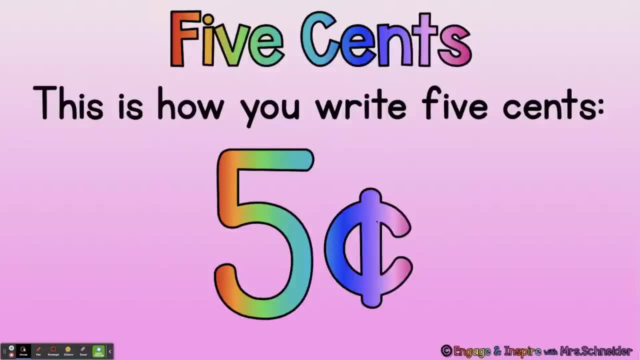 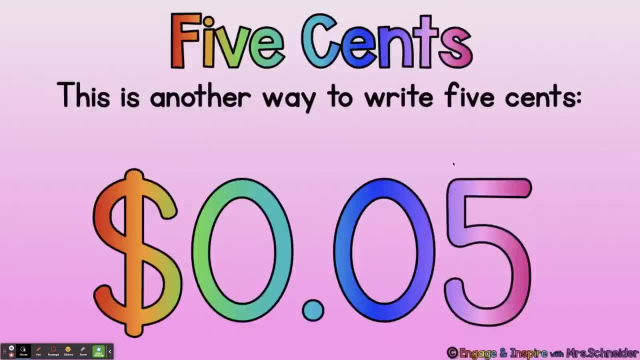 Draw a five in the air And then draw a C with a line through it That says five cents. This is another way to write: five cents: Zero dollars, decimal point zero: five Five cents. Counting nickels is the same as counting by fives. 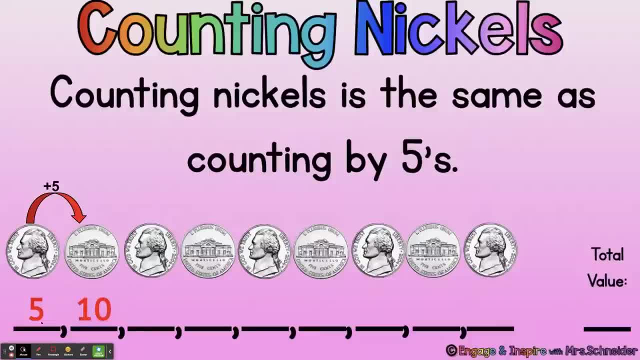 Five plus five is ten, So let's count by fives: Five, ten, 15,, 20,, 25,, 30,, 35,, 40,, 45. So these nickels have a total value of 45 cents. 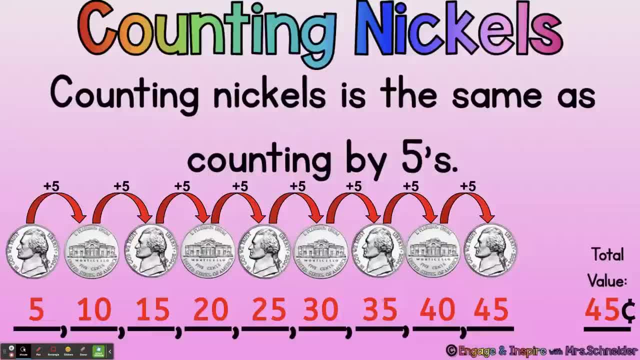 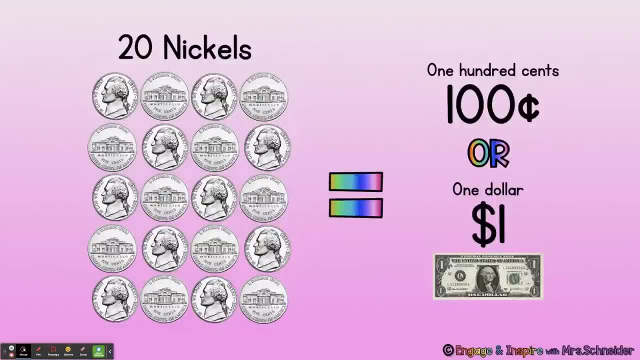 Can I buy anything with 45 cents? Hmm, I might be able to buy a couple of things, Maybe a pack of gum, 20 nickels- Let's count by fives and find out how much 20 nickels equals. Five ten, 15, 20,, 25,, 30,, 35,, 40,, 45,, 50,, 55,, 60,, 65,, 70,, 75,, 80,, 85,, 90,, 95, 100. 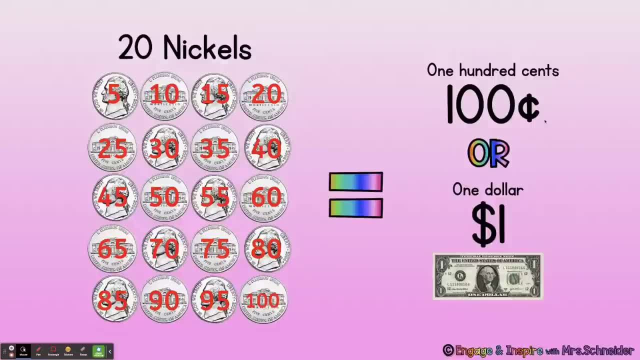 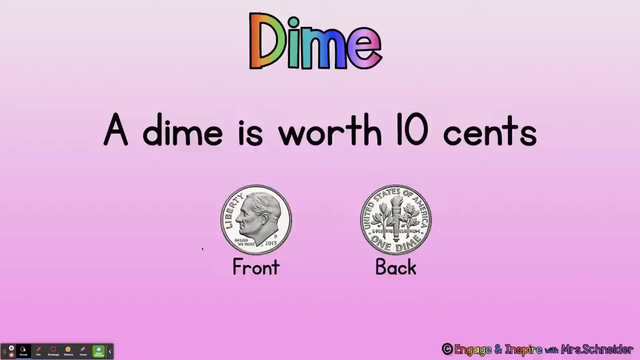 So 20 nickels equals 100 cents Or one dollar. 100 cents is the same as one dollar. So if I had 20 nickels I could trade it for a one dollar bill. A dime is worth ten cents. Here's the front of a dime. 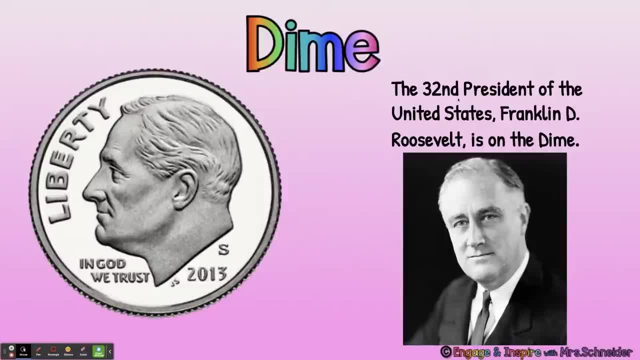 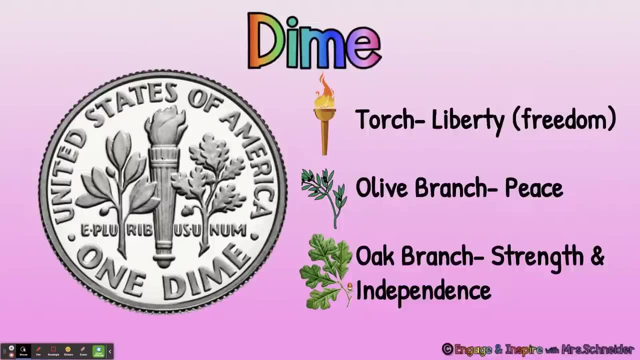 And here's the back of the dime. The 32nd President of the United States, Franklin D Roosevelt, is on the dime. Does that look like his picture? It's pretty accurate, I think. On the back of the dime you see a torch, which is a symbol of liberty or freedom. 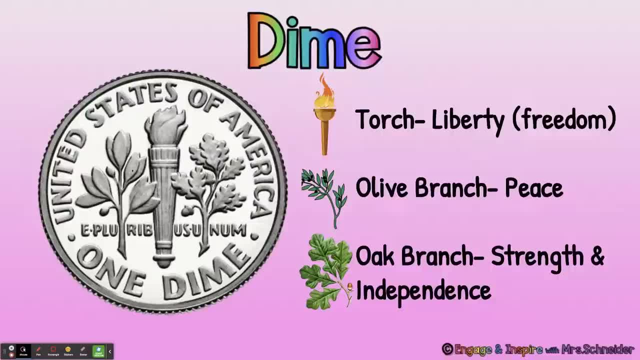 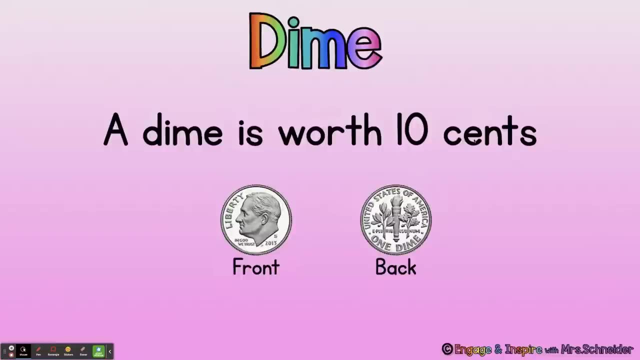 An olive branch right here, which is a symbol of peace, And the oak branch- see the little acorn- The oak branch, which is a symbol of strength and independence. A dime is worth ten cents. This is how you write ten cents. 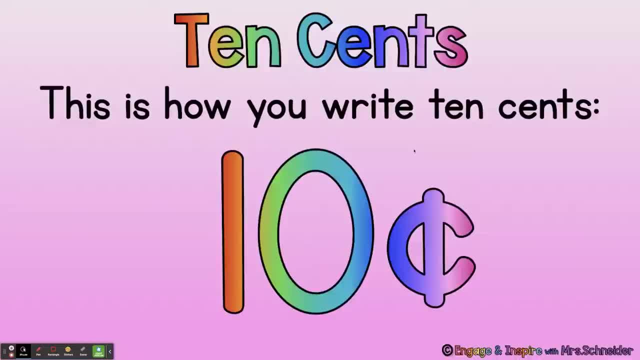 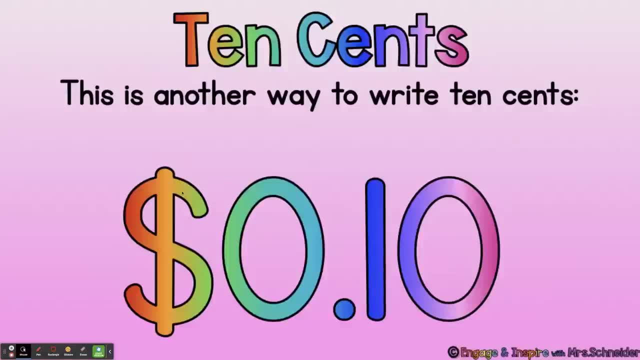 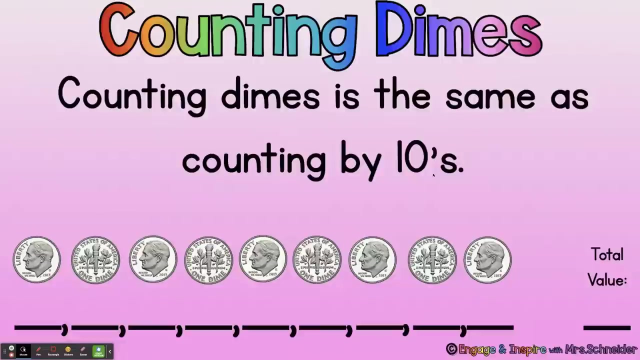 Draw it in the air: One zero and a C with a line through it: Ten cents. This is another way to write ten cents. Dollar sign: zero dollars, decimal point to separate the coins and ten cents. Counting dimes is the same as counting by tens. 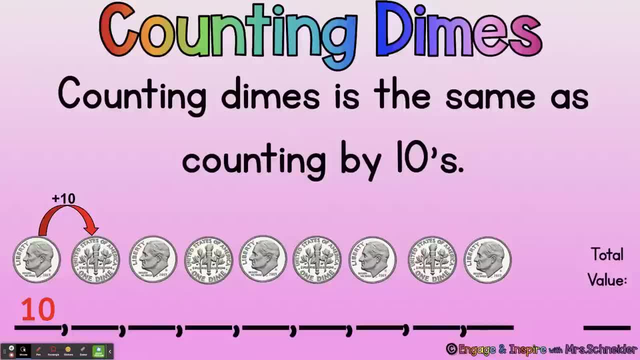 Let's count by tens. Ten plus ten would be 20.. So 10,, 20,, 30,, 40,, 50,, 60,, 70,, 80,, 90. So nine dimes has the total value of 90 cents. 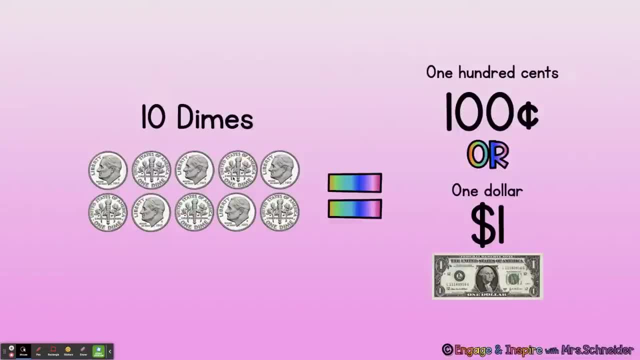 Let's see how much ten times equals Ten dimes: 10,, 20,, 30,, 40,, 50,, 60,, 70,, 80,, 90, 100.. 100 cents or one dollar. So if you find ten dimes, you can trade it in for a dollar bill. 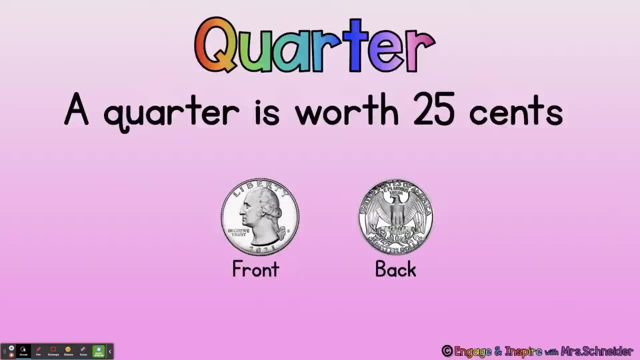 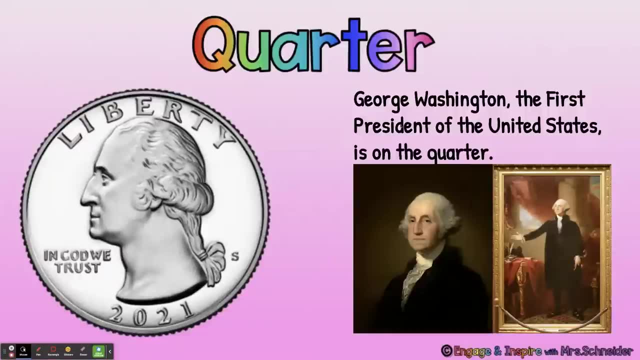 A quarter is worth 25 cents. Here's the front of the quarter and here's the back of the quarter. George Washington, the first President of the United States, is on the quarter. Here's another man with the long hair, And see, it has his curl there. 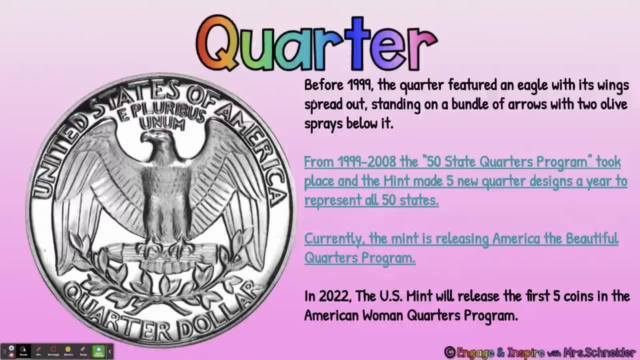 They captured that pretty well. So before 1999, the quarter featured an eagle with its wings spread out and standing on a bundle of arrows with two olive sprays underneath it. But from 1999 to 2008,, there was a 50-state quarters program. 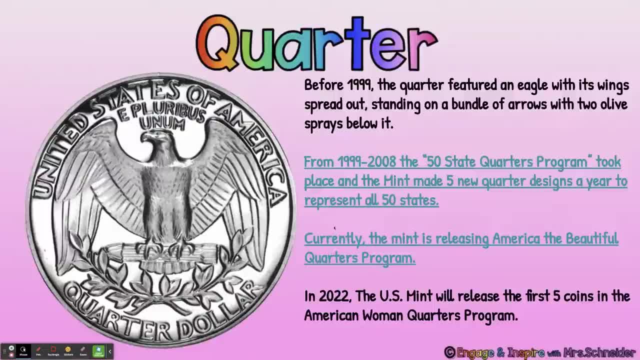 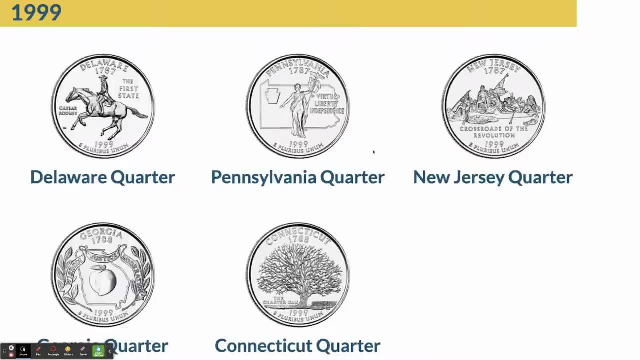 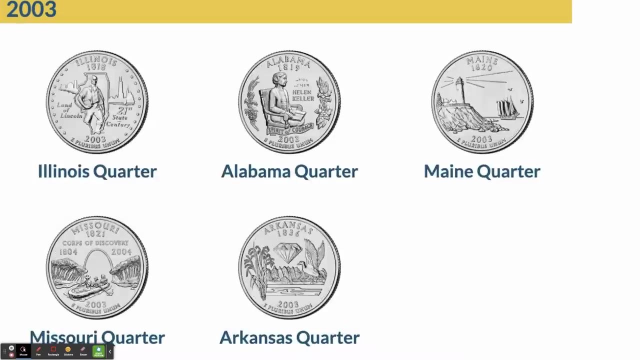 And so they made a bunch of different quarter designs. Currently, the Mint is releasing America the Beautiful quarter, And in 2022, they're going to release the first five coins of the American Woman Quarters program. Here's some of the quarters from the 50-state program. 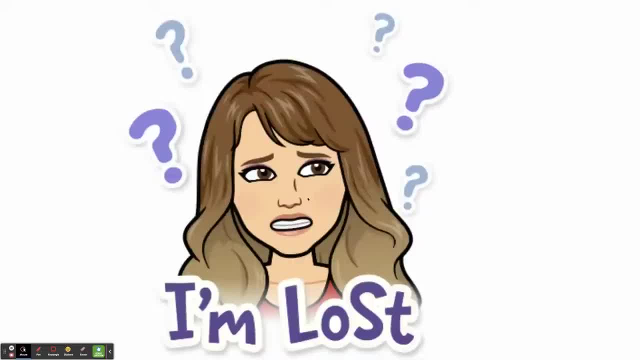 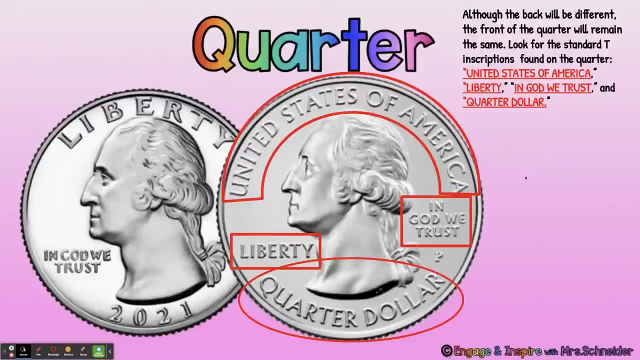 I know you might be feeling a little bit lost right now, Like with all of these different designs, how am I supposed to know what a quarter is or what coin it is? But although the back will be different, the front of the quarter will remain the same. 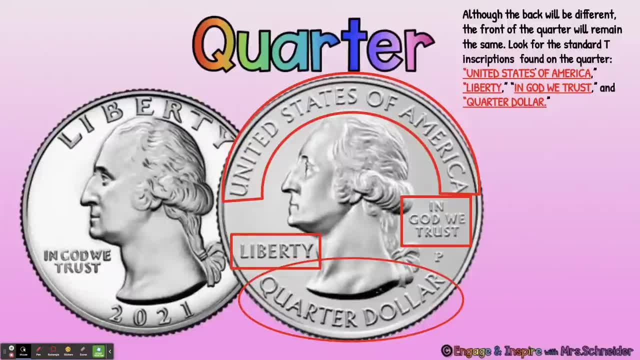 Or almost the same. Look for standard inscriptions found on the quarter Like: United States of America: Liberty. In God We Trust, Quarter dollar, And it will still have George Washington's picture on the front. So get to know that this is Mr George Washington, right here. 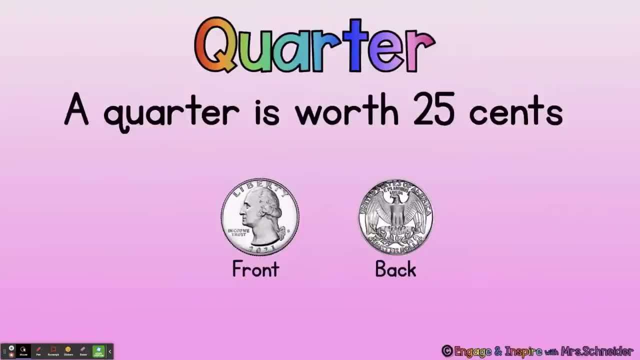 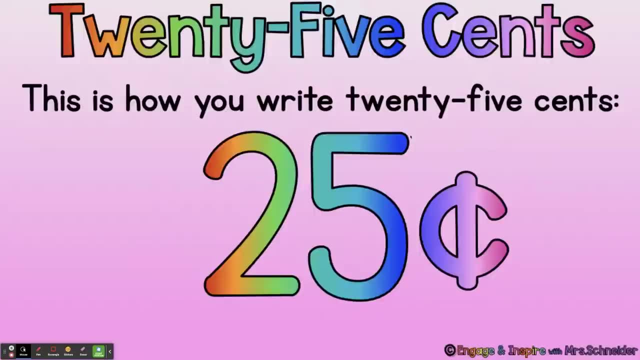 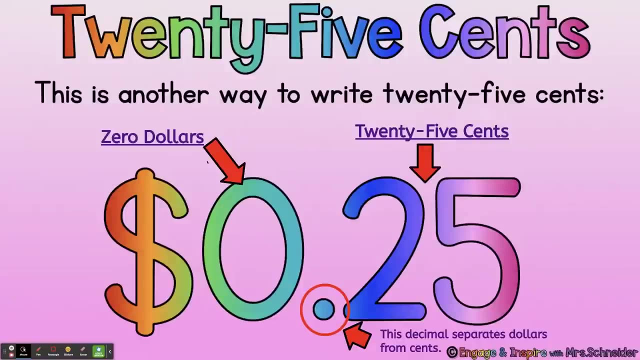 Same one. that's right here. A quarter is worth 25 cents. This is how you write 25 cents. Twenty-five cents: This is another way to write 25 cents. This is a dollar sign, So zero dollars And a decimal point to separate the change. 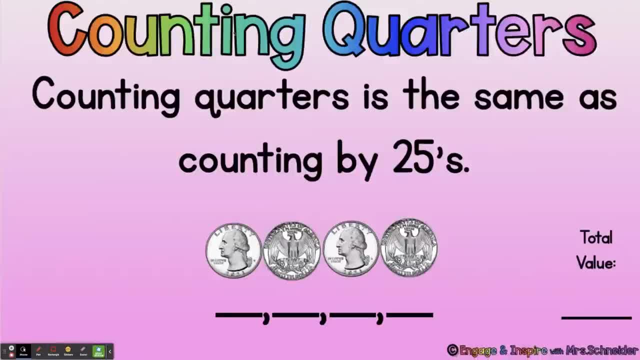 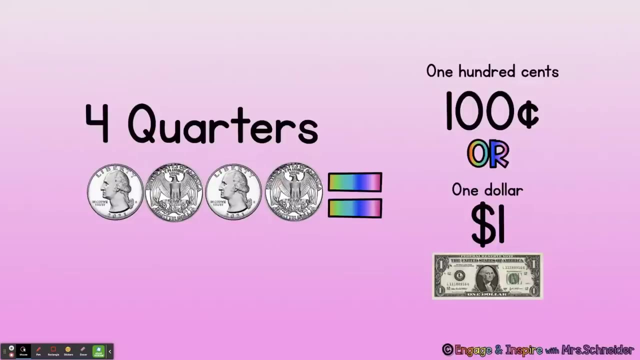 And 25 cents Counting quarters. Counting quarters is the same as counting by 25s: 25,, 50,, 75,, 100. So the total value of four quarters is 100 cents. Four quarters equals 100 cents, or one dollar. 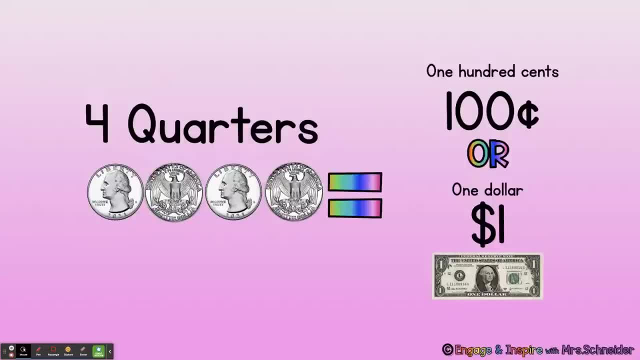 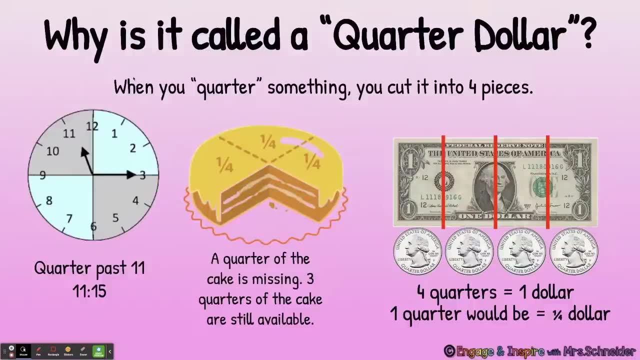 So if you find four quarters, you can trade it in for a dollar bill. Why is it called a quarter dollar? When you quarter something, you cut it into four pieces. So a clock is quartered. So this clock shows 1115.. 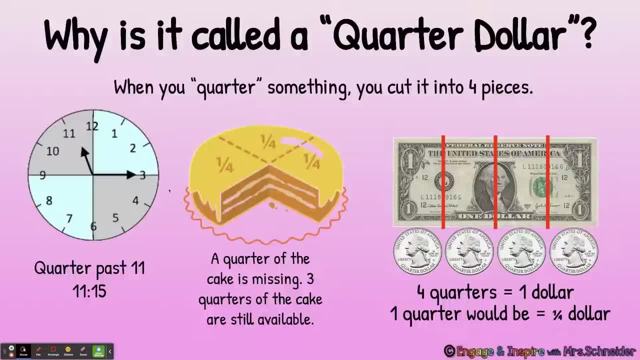 It shows one quarter past 11.. This cake is cut into quarters And there's one quarter missing And there's three quarters still available. A dollar is cut into four. So 25 cents plus 25 cents, plus 25 cents plus 25 cents is 100 cents. 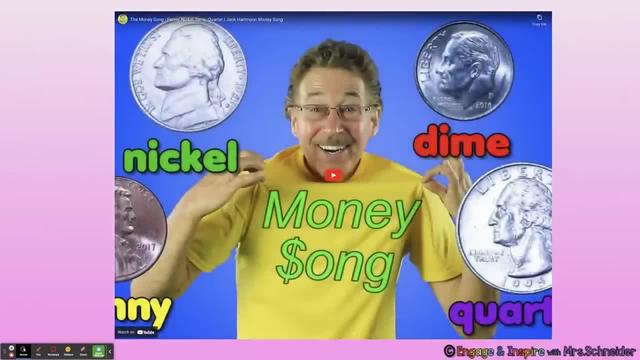 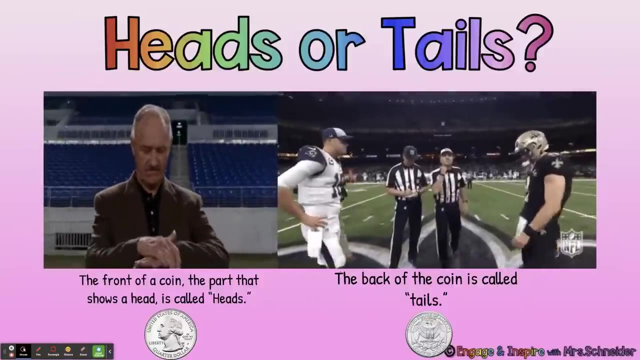 which is one dollar. Now is probably a really good time to get up and move. I really love this Jack Hartman video to dance along to the song and learn the names and values of the coins. Heads or tails: The front of the coin. 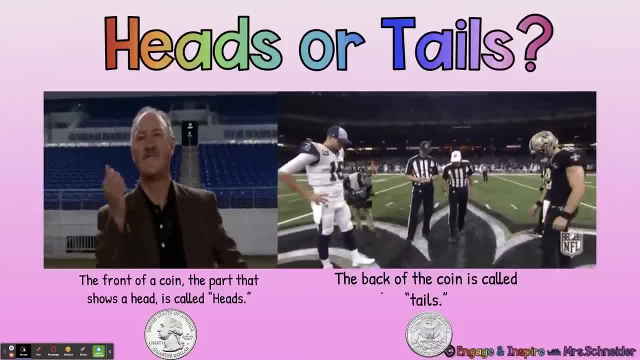 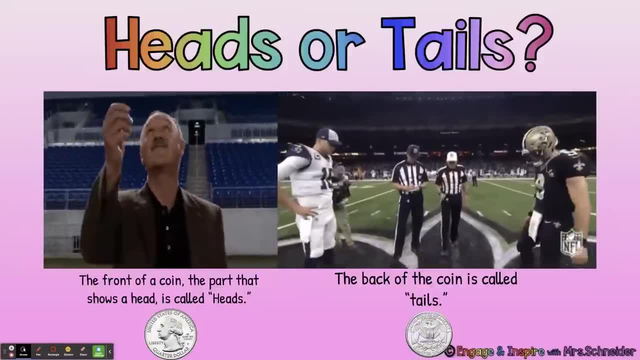 the part that shows a head is called heads. The back of the coin is called tails. So you'll see that at every football game they're going to toss the coin and say heads or tails And we'll see who the winner is. 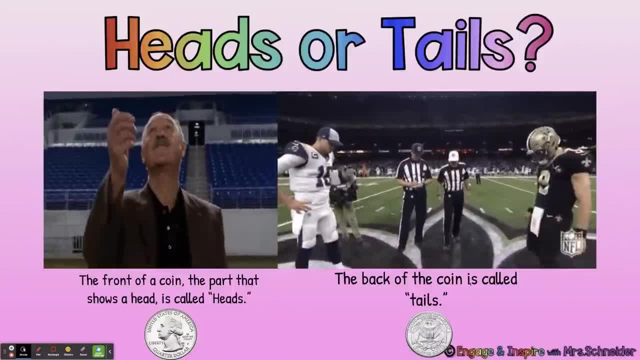 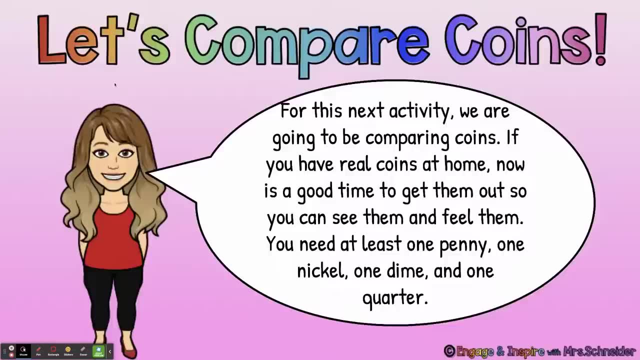 The person that guesses it correctly is the winner. Now comes the fun part For this next activity. we are going to be comparing coins. If you have real coins at home, now is a good time to get them out so you can see them and feel them. 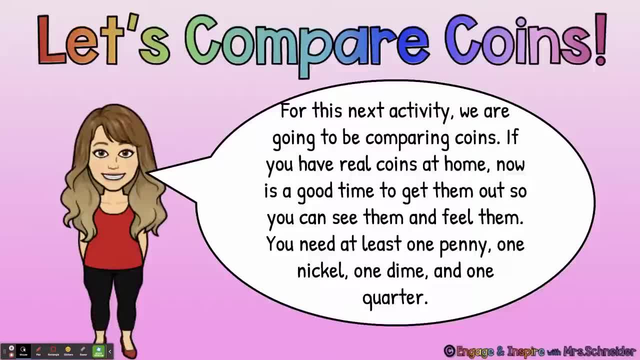 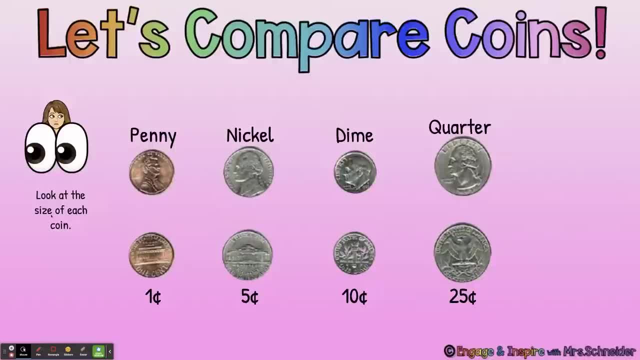 You need at least one penny, one nickel, one dime and one quarter. Let's compare coins. Look at the size of each coin: Penny, nickel, dime, quarter. Which coin is largest in size? Yes, the quarter is the largest in size. 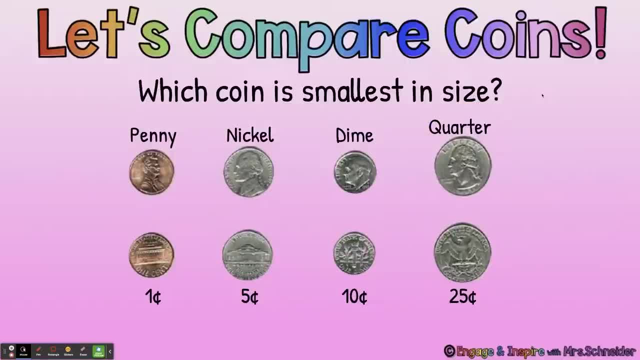 Which coin is smallest in size? Yes, the dime is the smallest in size, but not in value, right? Even though it's smallest in size, it's worth ten pennies. It is worth two nickels. It is worth a lot, even though it is the smallest in size. 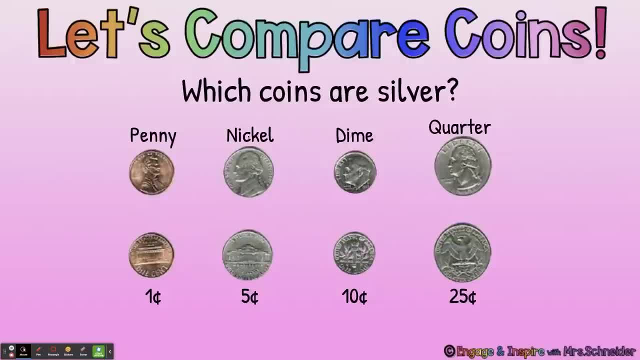 Which coins are silver? The nickel, the dime and the quarter. See how they all have that silver color. They're not made with real silver anymore. Which coin is not silver? The penny. The penny is a bronze-copper color. 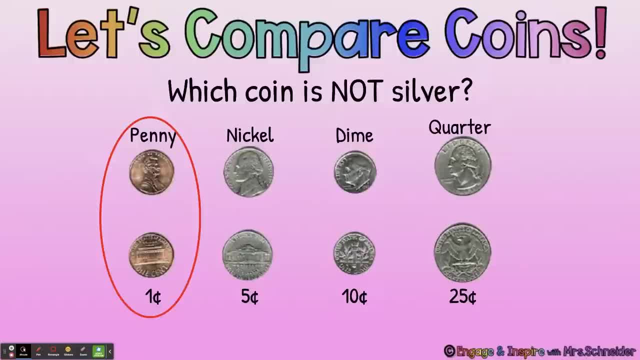 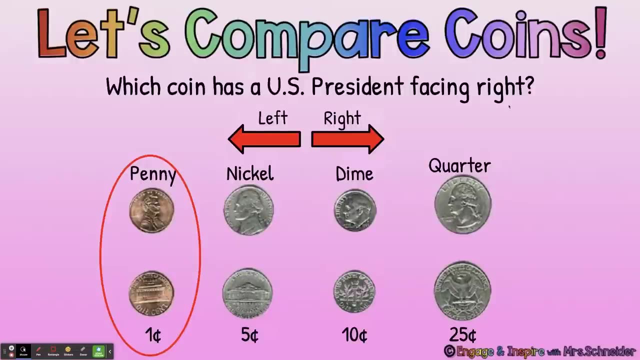 and when it's really clean and shiny it's more of a copper color, but when it gets dark, when it gets dirty, it's more. people usually call it brown. Which coin has a US President facing right? The penny? 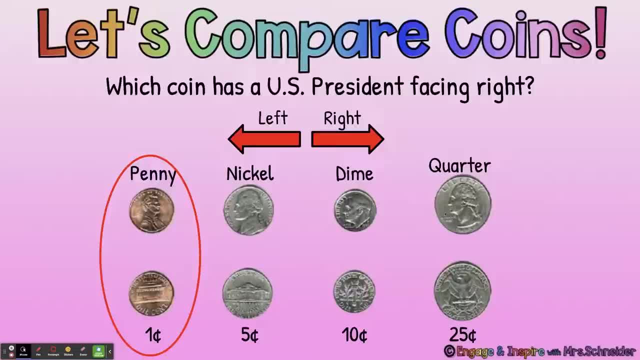 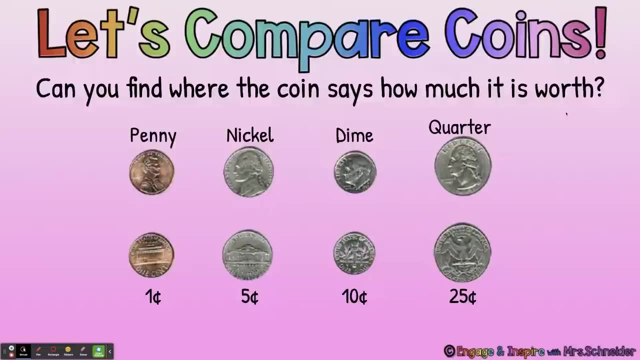 Look at all of these presidents are facing left, but Mr Lincoln is facing right. Can you find where the coin says how much it is worth Good eye? It says one cent. What about on the nickel? Can you find it? 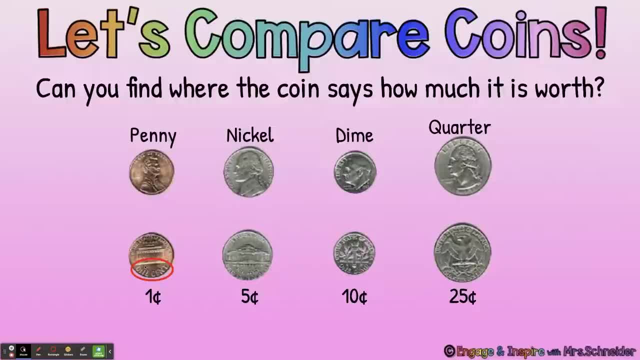 Yes, it is one cent. What about on the nickel? Can you find it? Yes, it says five cents. The dime says one dime. so I hope you know how much one dime is worth. It would be helpful if it said ten cents here. 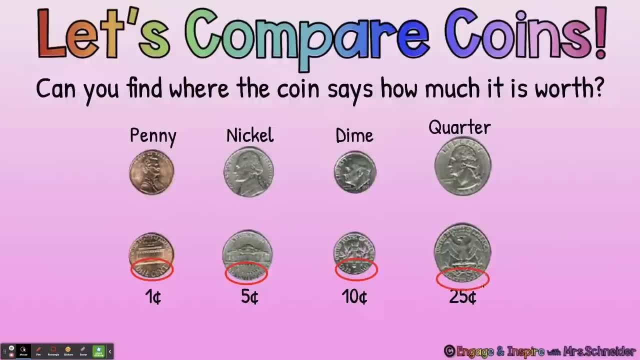 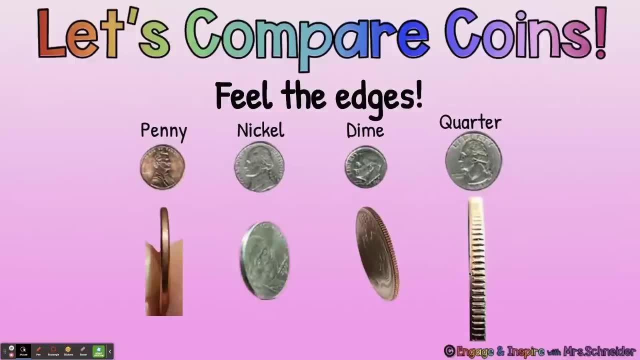 And the quarter says quarter dollar. to remind you that it's 25 cents, that it's a quarter worth 25 cents, Let's compare. Feel the edges. Feel the edge of the penny, Feel the edge of the nickel, Feel the edge of the dime. 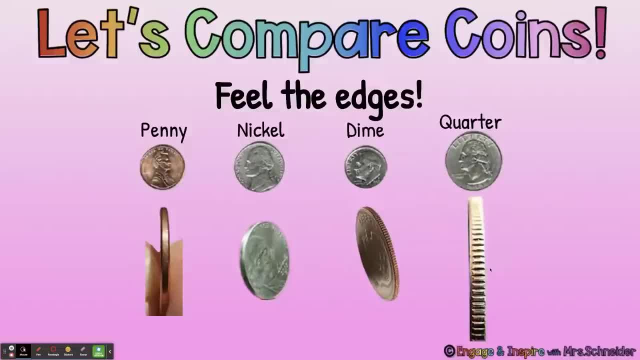 Feel the edge of the quarter. What do you notice? What are some observations? Which coins have a smooth edge? Yes, the penny and the nickel both have smooth edges. Which coins have a bumpy edge Or an edge with ridges? 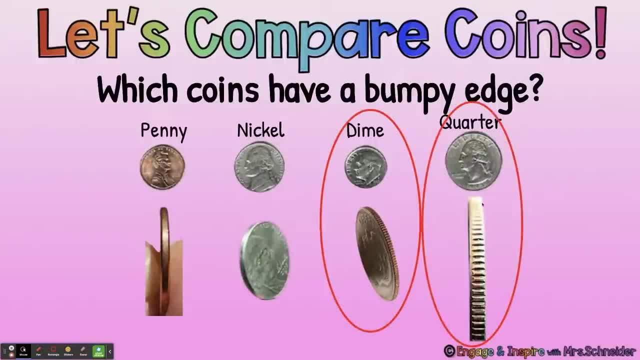 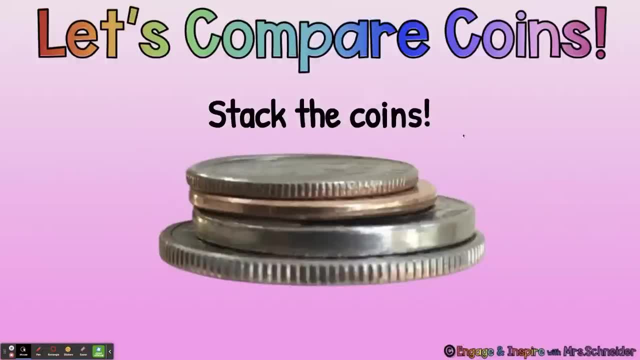 Yes, the dime and the quarter have ridges. See how they're not smooth. Now stack the coins. What do you notice? What are some observations you're making? What coin is on top? Why, The dime is on the top. 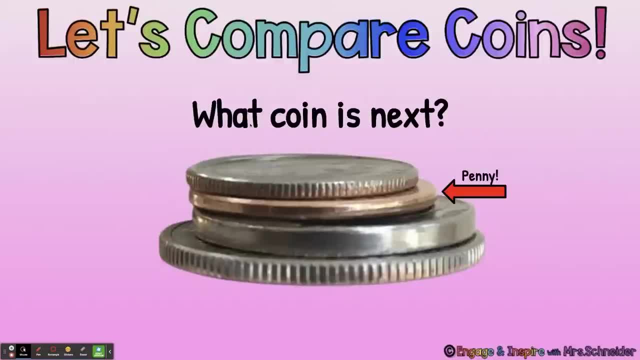 because it's the smallest in size. What coin is next? The penny, And what's going to be next? And look at how much thicker the next coin is than the penny or the dime. The next coin is the nickel, worth five cents. 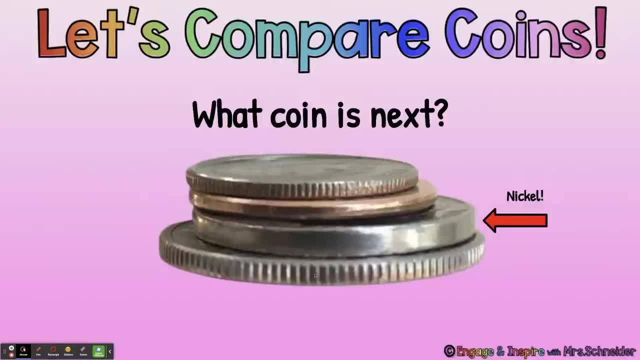 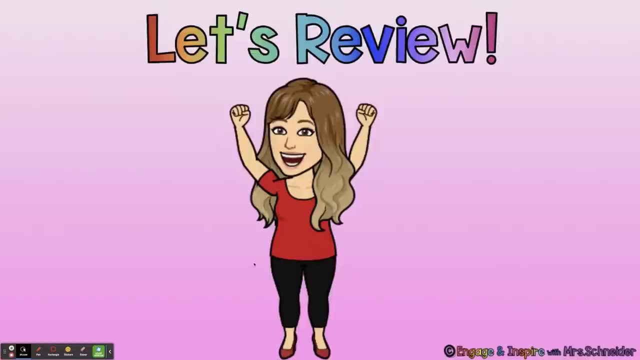 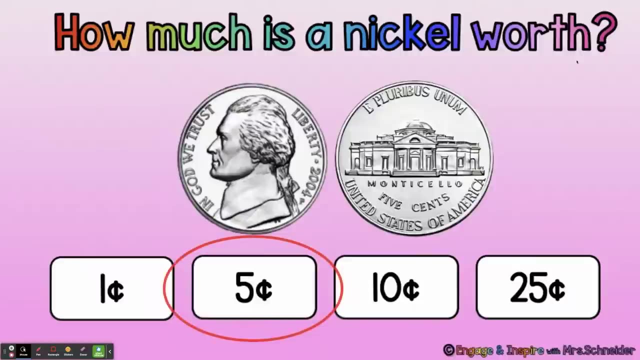 And the last coin with the rigid edges is the quarter, because it's the biggest. Yay, Let's review. How much is a nickel worth? Five cents? Good job. If you didn't know, the answer was right here. It said five cents. 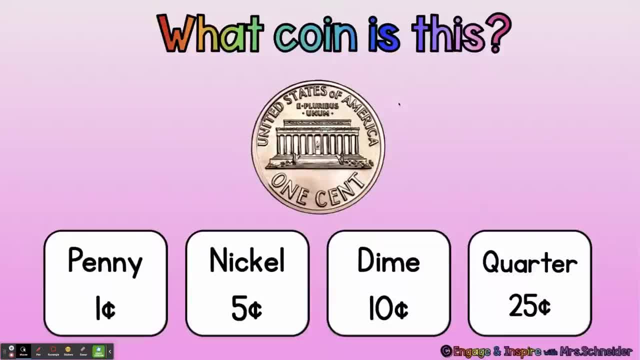 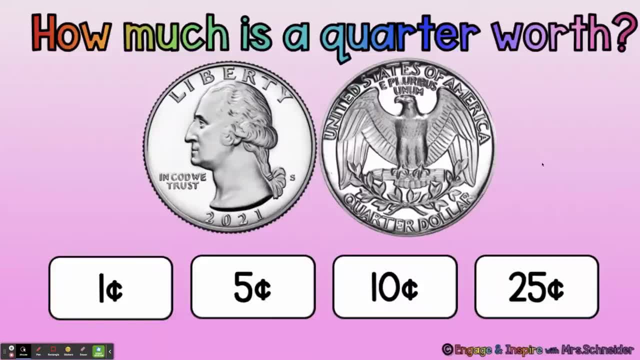 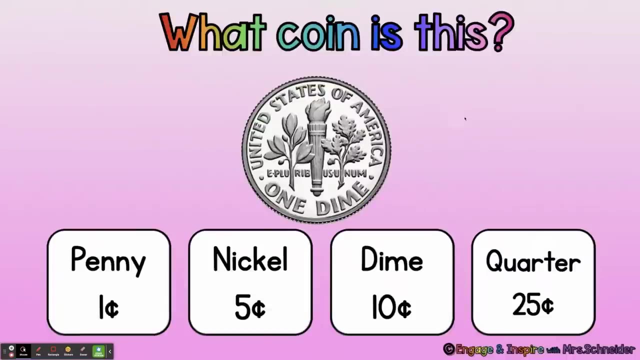 What coin is this? Yeah, it's a penny. It's worth one cent. How much is a quarter worth? Well, it's tricky because the answer's not on there. How much is a quarter worth 25 cents? What coin is this? 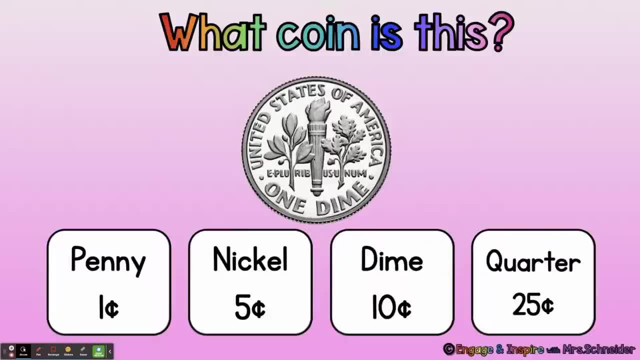 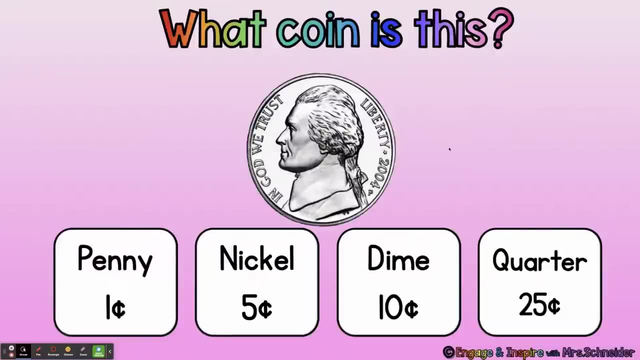 It has bumpy edges. It has the torch and the oak leaf and the olive branch. It's the dime worth 10 cents. See, It says dime right here. What coin is this? This one tricks a lot of people, but this one is the nickel.